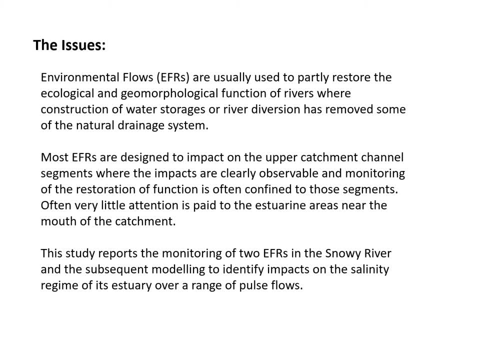 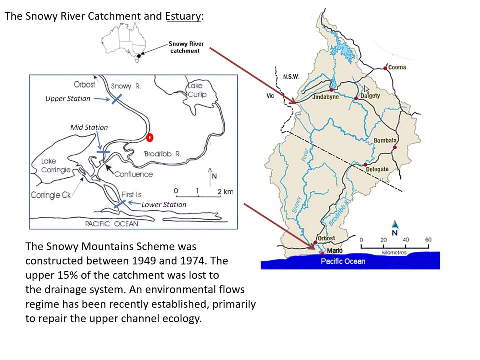 This study reports the monitoring of two environmental flows in the Snowy River and the subsequent modeling to identify impacts on the salinity regime of its estuary over a range of pulse flows. The Snowy River is an iconic river in Australia, the subject of poems, stories and film. 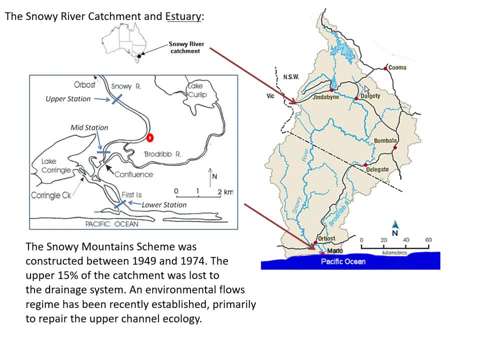 There's a long indigenous history and a far briefer history of European settlement, and is a recognized area of natural beauty. Despite this, it's only relatively recently that much attention has been paid to researching its function in any detail. The Snowy Mountains Hydro Scheme, constructed between 1948 and 1974, excised the upper 15% of the catchment above Jindabyne, as shown on the map to the right. 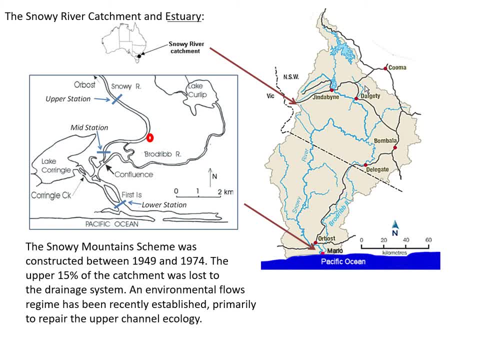 Altering the river regime for the rest of the catchment and the estuary, as well as producing a reduction in the magnitude of natural pulse flows. The spring snowmelt flow was almost completely removed from the main catchment. While some release of the snowy catchment was undertaken, it was piecemeal and far below that required to maintain the river in anywhere near its natural state. 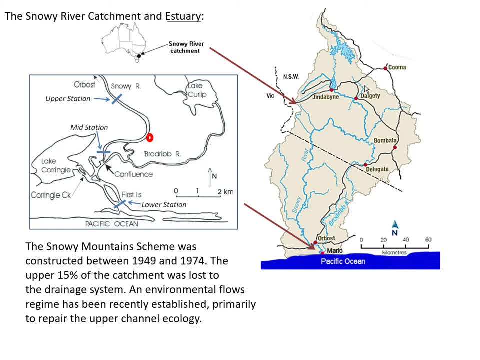 Over the last decade or so, an EFR regime has been established by various trial releases, including monitoring of the effects of the flows on the river. This regime has been designed primarily to repair the upper channel ecology and to hopefully mollify local concerns about the water quality of the river. 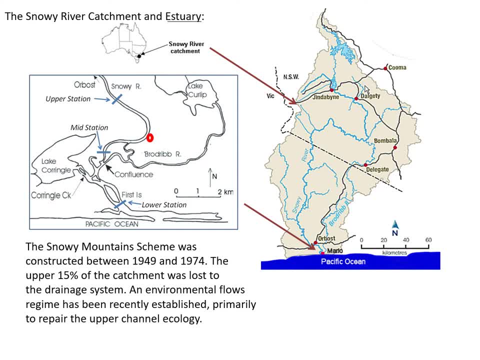 Note. on the map of the estuary. on the left of the slide, the upper, middle and lower locations mentioned in our modeling is marked in blue lines, as well as the red circle, which was our upper monitoring station for the specific flow releases we monitored and are depicted on the following slide. 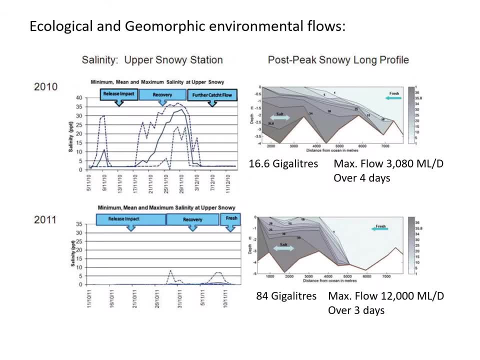 To explain the effects of EFRs of different magnitude, two pulse flows in 2010 were detected. The EFRs of 2010 and 2011 were monitored in the river segments of the catchment and, at this stage, John Hinwood and I offered to monitor the estuarine component of the system. 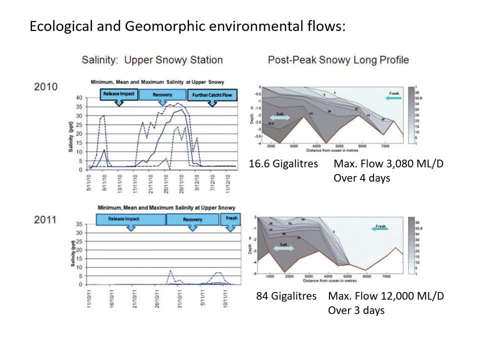 The 2010 EFR was designed as an ecological flow to reduce the impacts on the reaches below the dam, with some effects down through the catchment, while the 2011 EFR was a larger geomorphic flow designed to scour the upper degraded channels. From the figure we can see that the EFRs of 2010 and 2011 were monitored in the river segments of the catchment and at this stage, John Hinwood and I offered to monitor the estuarine component of the system. 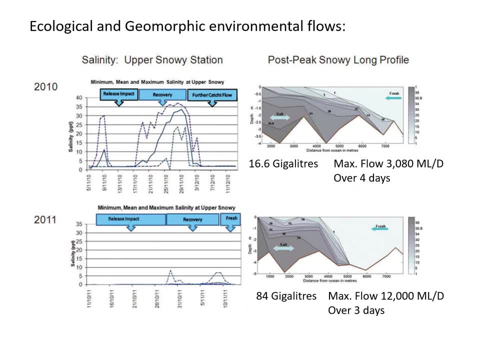 In terms the effects of EFRs with different magnitude. the figures on the right of the slide you can see the effects with the two flows on the salinity distributions in the estuary Immediate post-peak, with the displacement of the salt downstream differing, related to the different magnitude of the EFR flows. 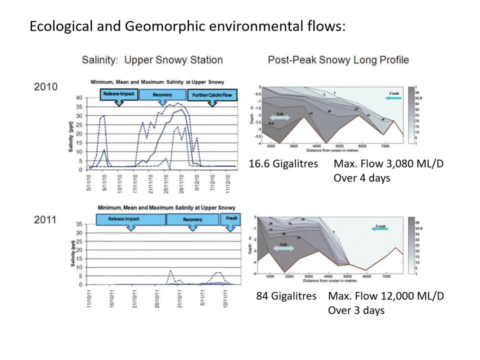 The figures on the left of the slide show time histories of the salinity at the upper monitoring station. The impact was obviously different for the two flows of different magnitudes. its struggling everytime is: recovery is expected for a long time. not a good time�. cuestions later can be observers for too much lad lad. 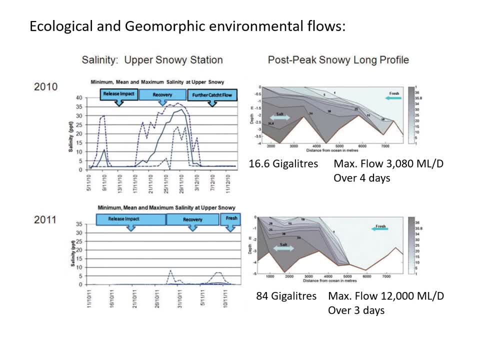 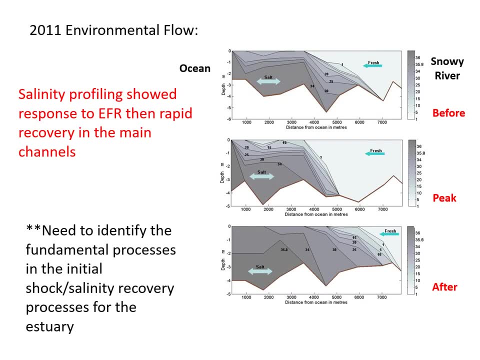 the salinity patterns, obviously making our job more difficult in extracting data for an empirical evaluation of pulse flows. this slide picks up on the downstream variations in the impact of the 2011 vfr on the salinity distribution, with the profiling before peak and after, illustrating the shock recovery patterns. 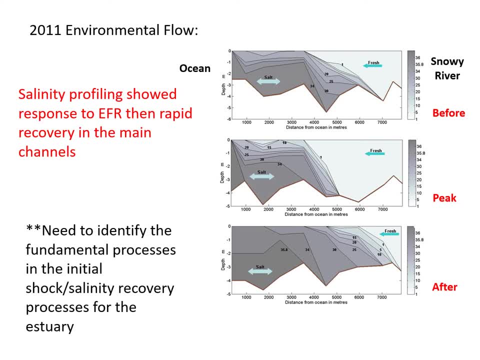 at time stamps during the release. the important thing to realize at this stage is that a purely empirical study is not feasible and that some modeling is required to look at the fundamental processes over a range of different flow magnitudes and durations, where we can control the model inputs to exclude interruptions by other natural 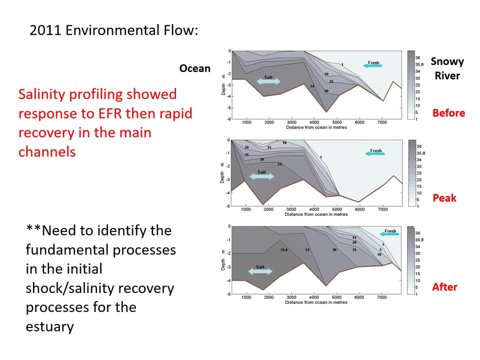 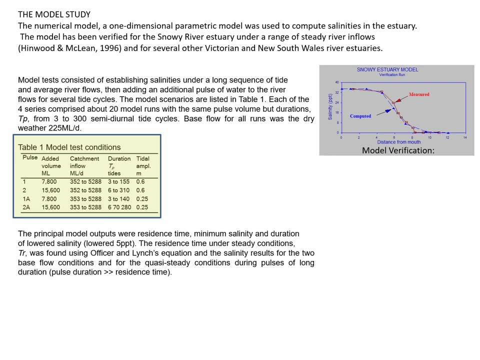 flows. this would permit examination over a selected range of flows that might be within the budget and limited water resources of the management authority. we used our established model, which has been reported elsewhere and is referenced in the top text on the slide. it is a numerical model, a one-dimensional parametric model. 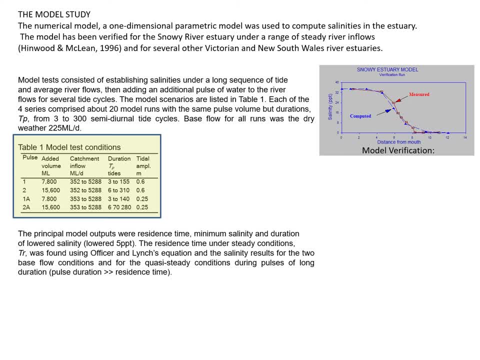 and we use that to compute the solidities in the estuary. the model has been verified for the snowy river estuary and the verification is shown on the right of the slide, giving quite an adequate representation of the measured salinity. it's also been applied to several other victorian new south wales river estuaries. 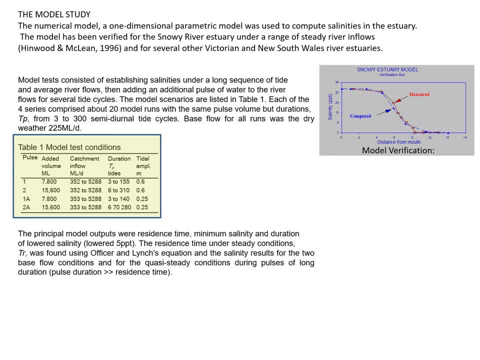 with the same sort of success. the model tests we use consisted of establishing salinities under a long sequence of tide and average river flows and then adding an additional pulse of water to the river flows for several tide cycles. the model scenarios are listed in table one which is highlighted in the middle. 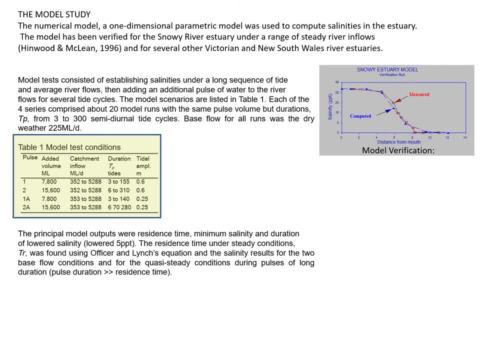 of the slide. each of the four series comprised about 20 model runs using the same pulse volume but durations ranging from three to three hundred semi-dynamal tidal cycles. the base flow that we used for all runs was the dry weather value of 225 megaliters per day. you'll note also that we use two. 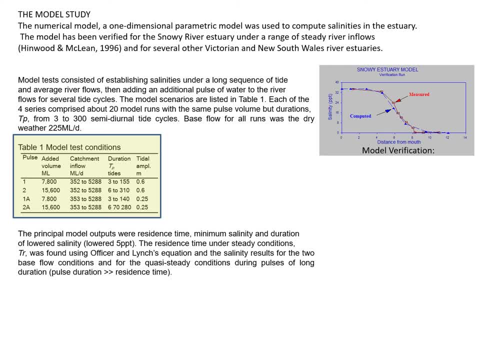 different tidal amplitudes, representing, in the case of 0.6 meters, the open estuary or the open entrance to the estuary, and the 0.25 where the entrance was constricted. the principal model outputs were residence time, minimum salinity and duration of lowered salinity. 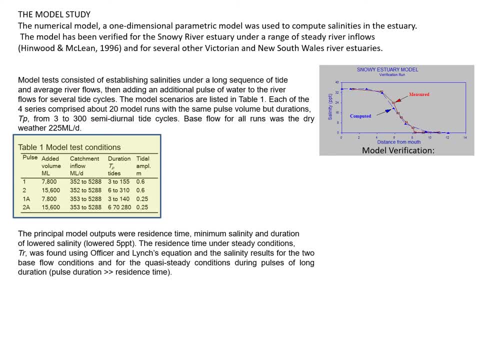 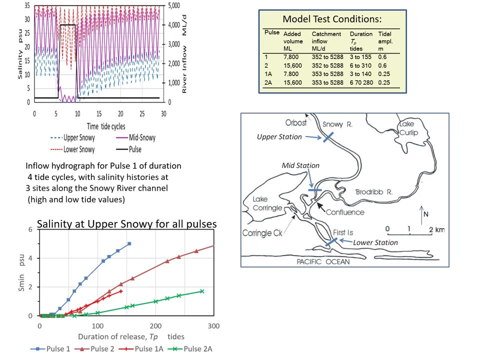 the residence time under steady conditions. we used uh offer, sir and lynch's 1981 equation and the salinity results for the two base flow conditions and for the cause of quasi-steady conditions during the during pulses of long duration. this next slide illustrates some of the model results. 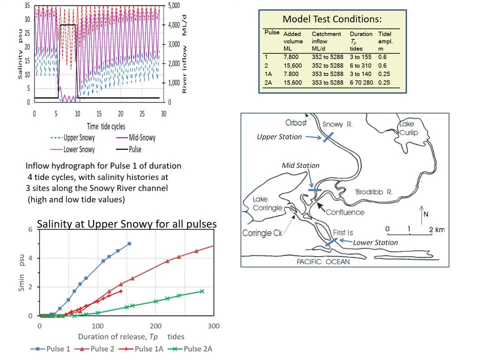 in the upper left of the slide you can see a plot of one of the pulse examples for pulse one, this one running for only 30 tides. the ambient salinity and tile variations for each of the stations is shown to the left of the solid black line depicting the pulse. 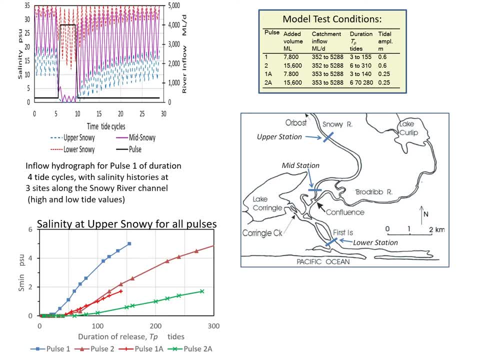 the pulse impacts over time are clearly seen with most variation, both tidally and also in magnitude and magnitude of the pulse. the pulse impacts over time are clearly seen with most variation, both tidally and also in magnitude, and also in magnitude of the pulse occurring at the middle station. 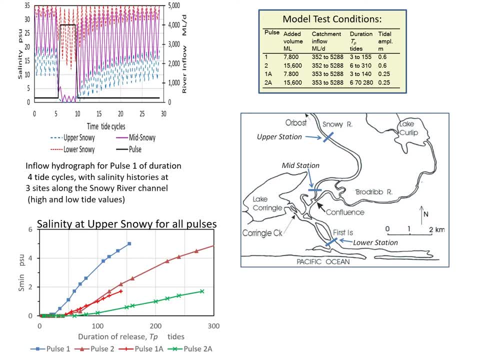 The recovery extends over the 30 tides here without reaching ambient salinity levels. Separate runs were made with the same total volume for each pulse, but with varying durations and the tide range selected from the two examples. The top left graph is just an illustration of one of those runs. 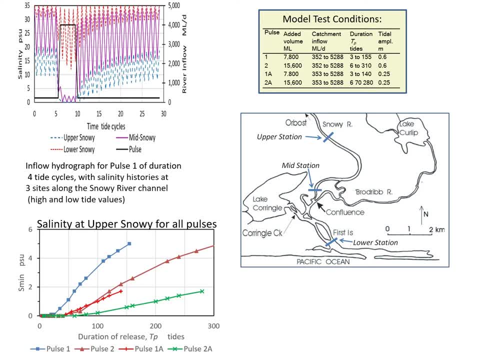 The bottom left graph summarizes these runs, with the x-axis showing pulse duration and the y-axis the minimum salinity observed during or following the pulse. While this graph shows significant variation due to pulse length, it's possible to further examine the results using a scaling technique. 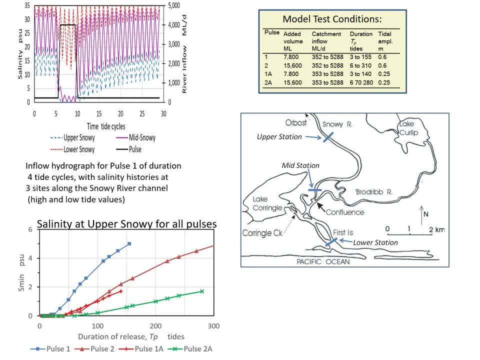 to systematize the data. From our analysis, and confirmed by trial, we've established that the parameter that best collapses the data is what we call the estuary flushing parameter, explained in the next slide. This is a measure of the ratio of the volume of water in the estuary. 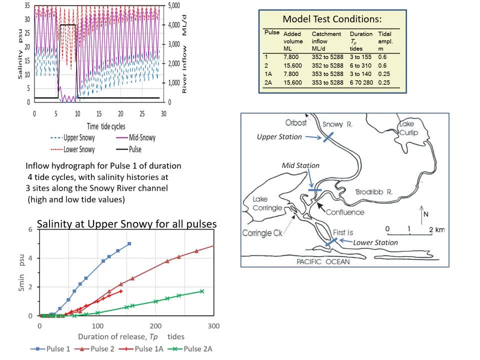 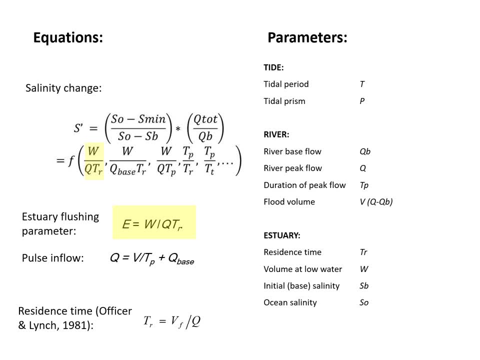 to the inflation rate. This is the flow from the catchment in a time relative to the flushing time. This slide is included for your future reference and contains, on the right-hand side of the slide, the parameters used for the tide river and estuary in our modeling. 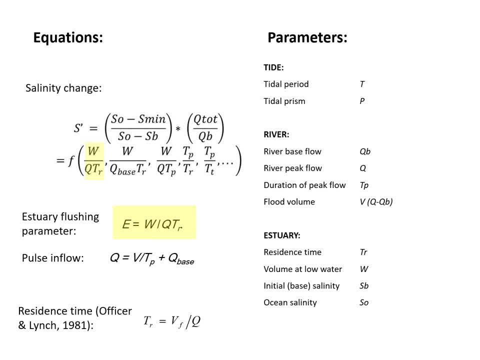 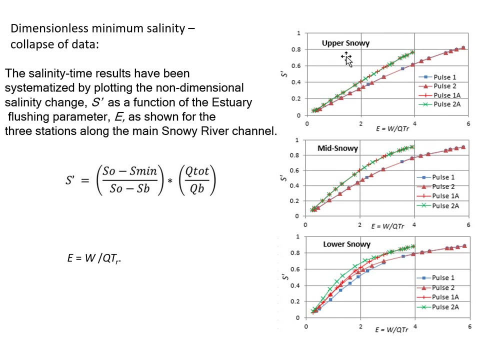 From the list of equations on the left, you can see that for the salinity change, we have extracted a ratio that forms the estuary flushing parameter, which is highlighted in yellow. Scaling techniques are often used via dimensionless equations to generalize problems, since dimensional analysis is the solution. 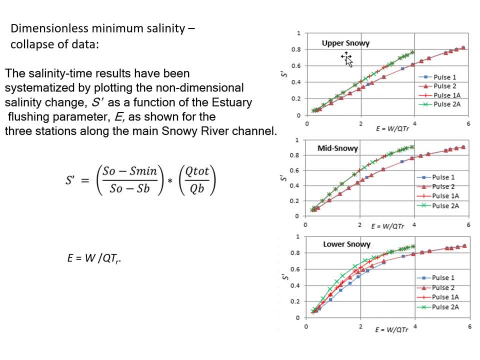 for a particular problem and we're looking for relevant variables to describe the patterns in the data that reveal the characteristics of the system. We found that by using the estuary flushing parameter, shown again here at the bottom left of the slide, we could collapse the results. 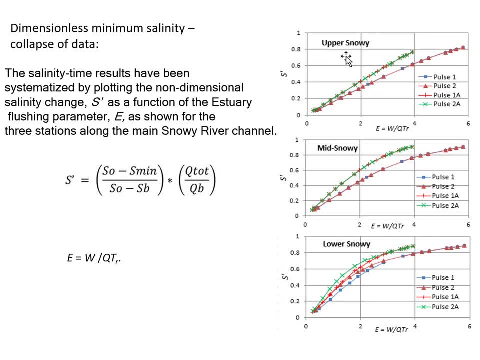 to illustrate significant relationships. The salinity time results have been shown in the following slide. The salinity time results have been systematized, then, by plotting the non-dimensional salinity change S prime as a function of the estuary flushing parameter E, as shown for the three stations.